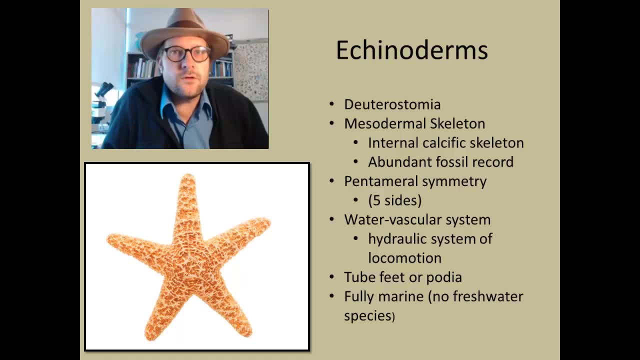 group of invertebrates that we are examining in this class that are members of the Deutostomia, That is, that they are actually more closely related to us than any other invertebrate that we will look at in this class. Echinoderms include Yellowtail, Sea Cucumbers, Sand Dollars. 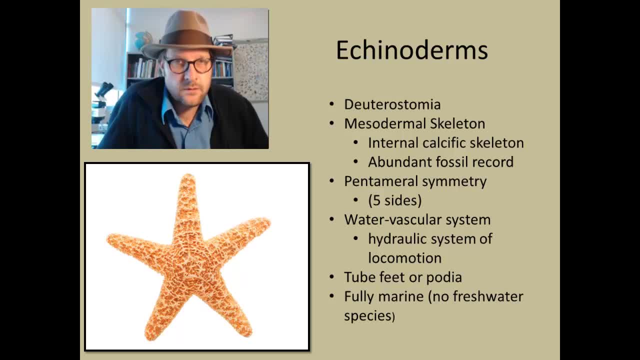 and all are marine invertebrates living within the oceans of the world. Echinoderms exhibit a mesodermal skeleton of porous calcite that can be covered by a spiny skin. Many exhibit a 5-point symmetry, or pentamere symmetry, with other groups, usingAScensir to suppose. 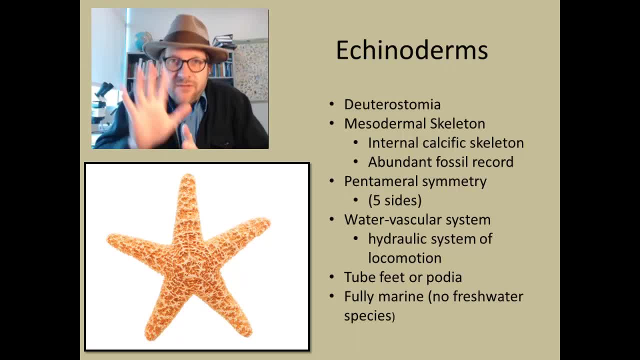 a more bilateral symmetry. This unique 5-point symmetry is found in many fossil groups and is a good way to recognize this group in the fossil record. Echinoderms rely on a very complex water vascular system, which is a hydraulic way of moving. 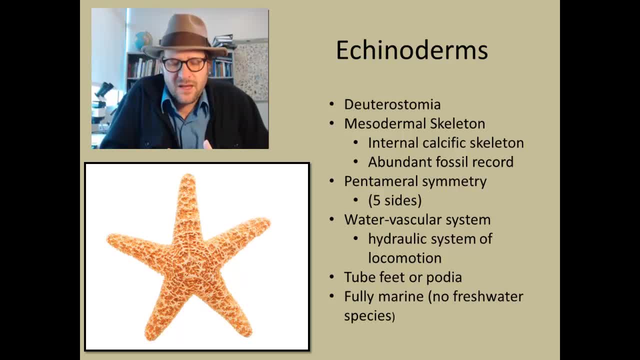 and it is a very strong and effective locomotion. This is therefore very different from the tendons and ligaments which run through serrated muscle, like in our own body, That muscle tissue can only contract. This water vascular system is much stronger than muscle action because the fluid is pumped. 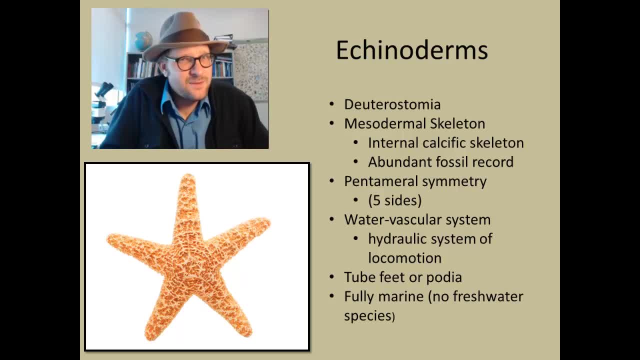 into different parts of the echinoderm's body and can be really strong when it comes to crushing strength. Unfortunately, with a water vascular system for locomoting, it has a significant downside, and that is that the water regulation must be achieved using water with a consistent 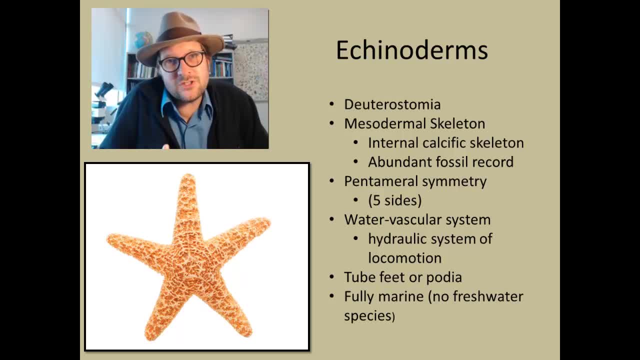 amount of salinity. So if you have too much or too little salt in the water, it can cause the water to flow through the cellular membranes and shifts in salinity can be deadly to echinoderms, since it disrupts their water vascular system. 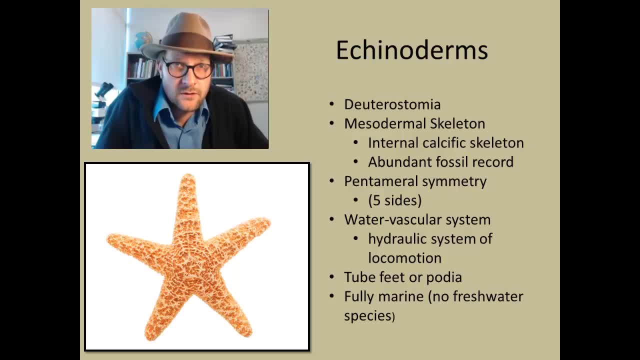 As such, echinoderms have never transitioned into fresh waters. Echinoderms are stellohyaline, which means that they are only found in ocean waters with a consistent salinity. The hydraulic water vascular system feeds into a large network of tube feet or podia. 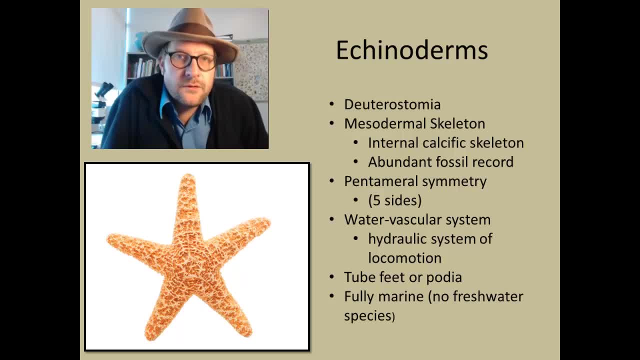 that emerge on the outside of the skeleton through numerous pores. These tube feet move back and forth, allowing the echinoderms to crawl slowly across the ocean surface, but they are also incredibly strong for cracking open shells. Echinoderms are also very strong for cracking open shells. 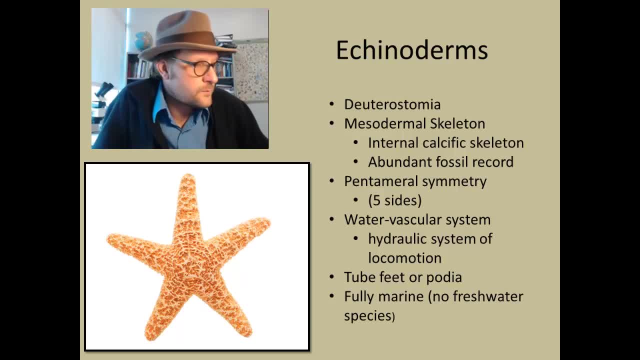 Echinoderms are also very strong for cracking open shells, And many echinoderms are significant predators on shelled organisms like bivalves and brachiopods. Because echinoderms have a calcitic skeleton, they are very common in the fossil record. 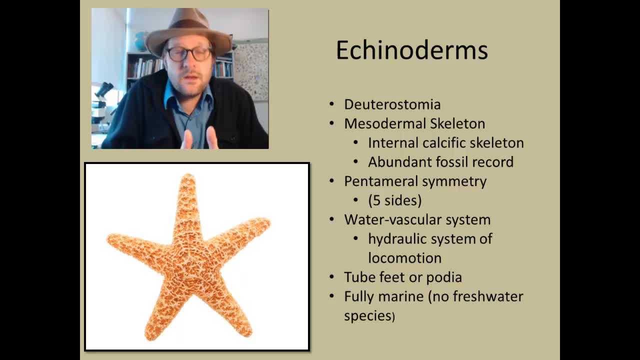 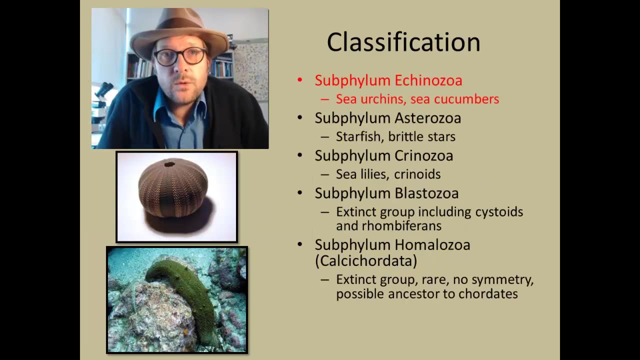 beginning in the Cambrian and become more diverse through time. In fact, today echinoderms are extremely diverse, with only two groups which are totally extinct. Alright, the major groups of echinoderms. The first subphylum is the Ichneozoa, which includes sea urchins and sea cucumbers. 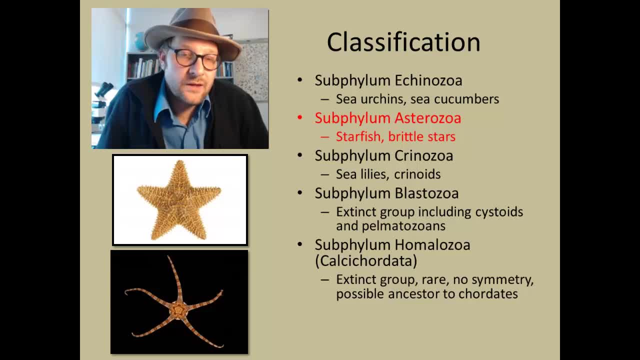 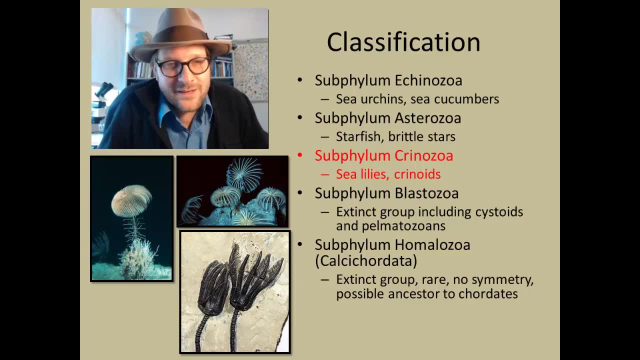 The second subphylum is the Astrozoa, which are the starfish and brittle stars. The third subphylum is the Cryozoa. these are the sea lilies and crinoids, a very common group in the fossil record. 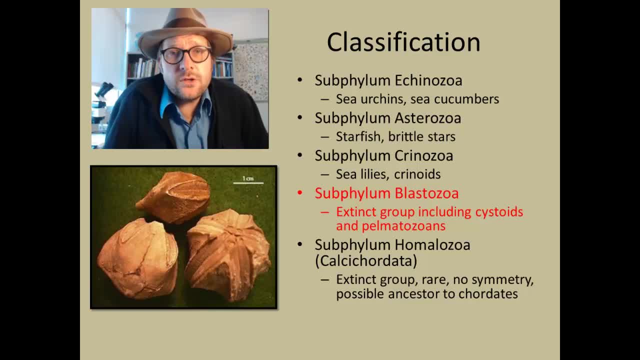 And the fourth group is the subphylum Blastozoa, which includes Cystoids and Raminiferins, which may be a new group to you, since the Blastozoa all went extinct at the end of the Permian and is the first subphylum that is totally extinct. 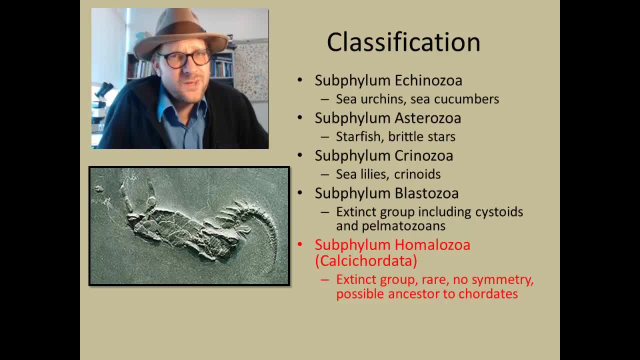 The fifth and final group of the echinoderms is another totally extinct group, the Homeliozoa, also known as the Chalcocordata. These fossils are… Really weird since, unlike other echinoderms, they do not have a five-point symmetry, or 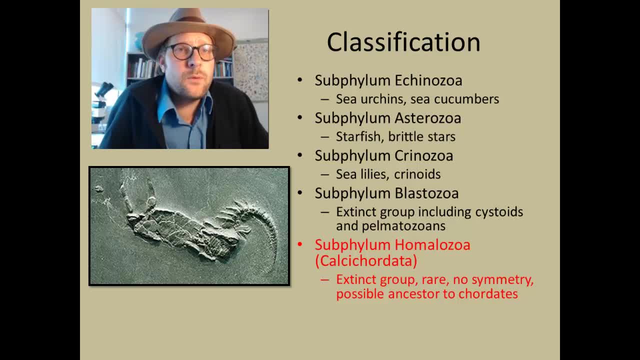 even a bilateral symmetry. A few scientists have proposed that they are related to chordates, their vertebrates, but this group exhibits a skeleton composed of calcite which is not like other chordates. The calcite skeleton is much more similar to what we find in echinoderms, and so they 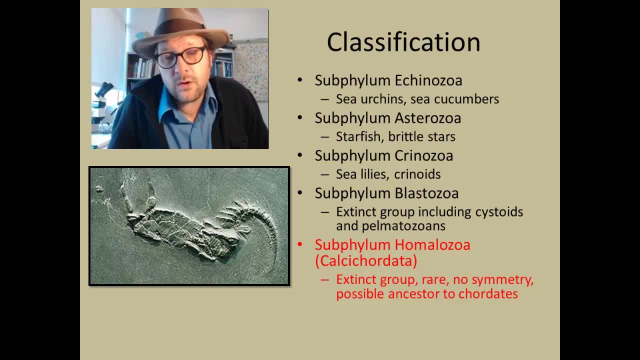 are often placed within echinoderms. So they are often placed within echinoderms. They are only known from the early Paleozoic, having gone extinct during the Devonian. So let's look at each one of these groups in more detail. 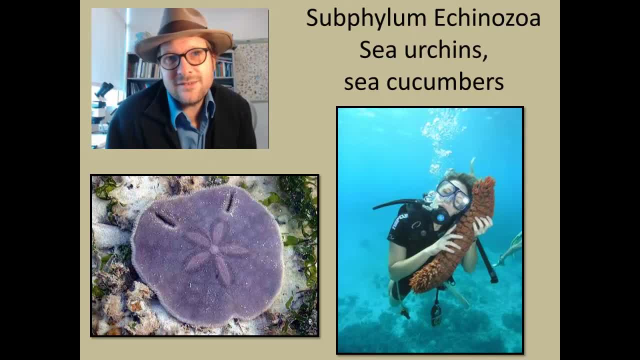 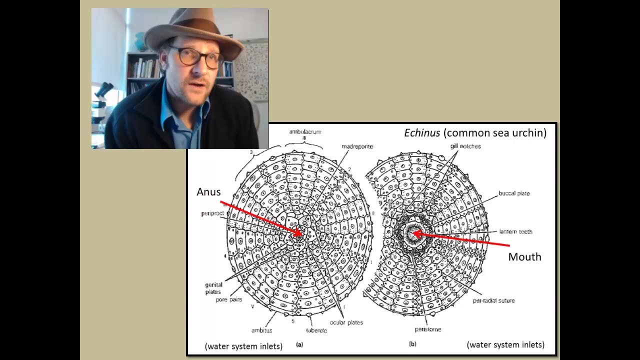 The Echnozoa include the sea cucumbers and sand dollars and heck, let's face it, they are kind of cute and cuddly, if not a little pokey. Animals that closely resemble the common sea urchin Echnodes have a very extensive fossil. 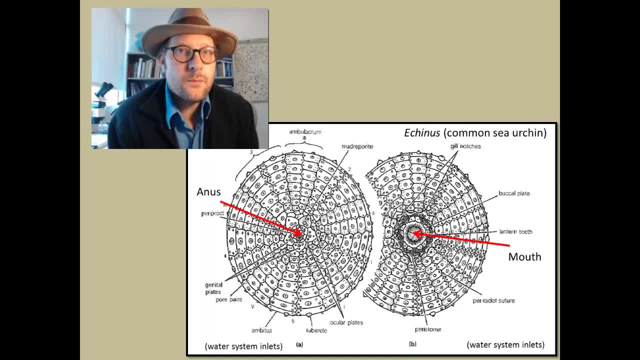 record. Their skeletons, preserves and bones are found in the Echnozoa. In the Echnozoa there is an opening for the mouth near the seafloor surrounded by gill notches, and an anus above surrounded by genital openings that release sperm or 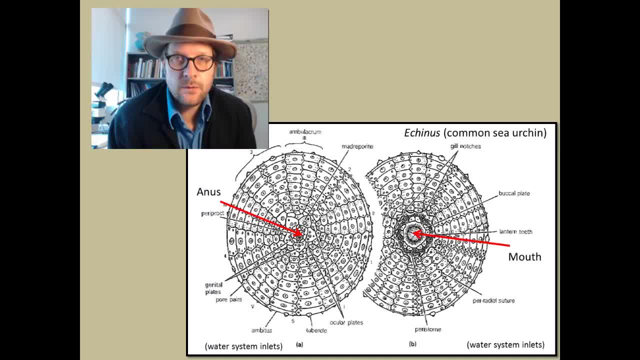 egg cells. A gut tube extends through the center of the animal. Each pore in the skeleton called a test is for the water-driven tube feet that extend through those pore openings and can retract when fluid is withdrawn from the feet, In particular at the bottom surface that is in contact with the ocean floor. 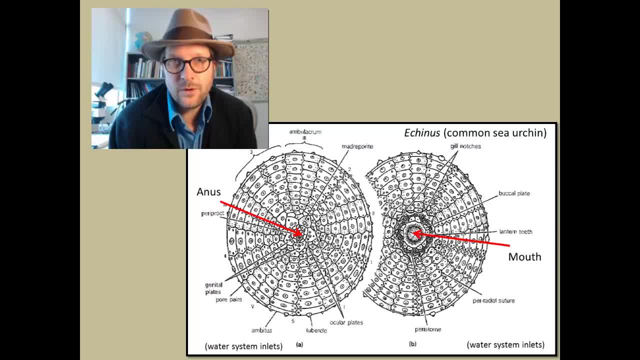 Not many lives are exposed by this tube. so, to be fair, not many know the reality of the Echnozoa. From a beauty perspective, Echnozoa is a very interesting species. One of its most remarkable features is the masculine apparatus called Aristotle's. 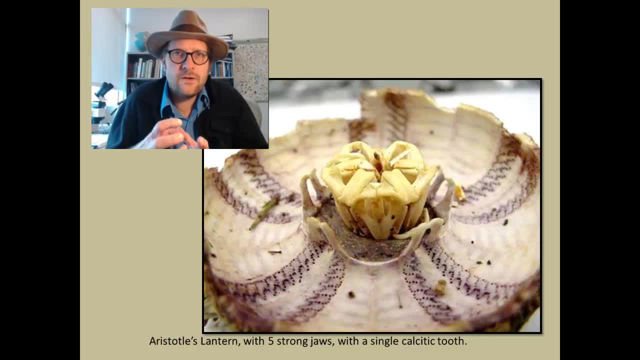 lantern, which is an arrangement of five strong jaws, each with a sharp calcitic tooth. The system is driven by a pyrognathic girdle that draws the teeth together to rasp or scrape at food, which is then passed down the gut tube through the body of the echinoderm. 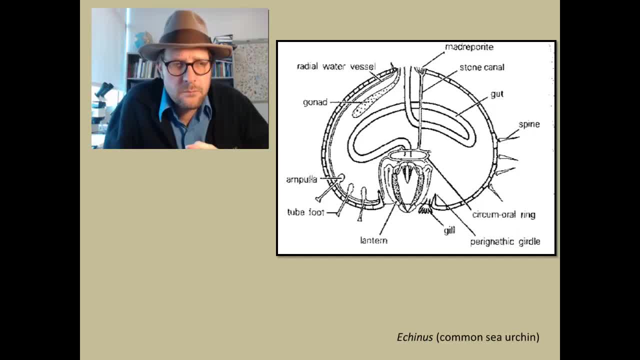 The inside of the test or skeleton is rather sparse, without many organs. besides the gonads which greatly inflate during breeding to release either eggs or sperm into the water. for external fertilization, The materporite serves as an opening for the water vascular system through a stone canal. 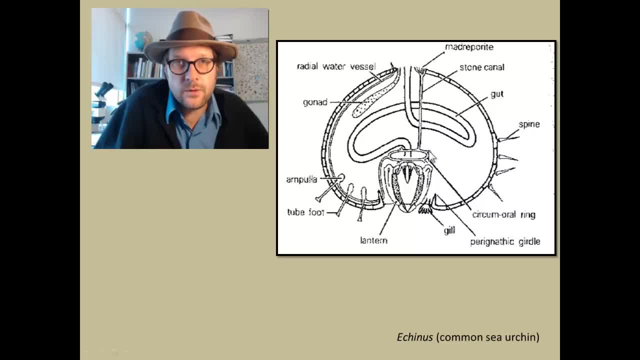 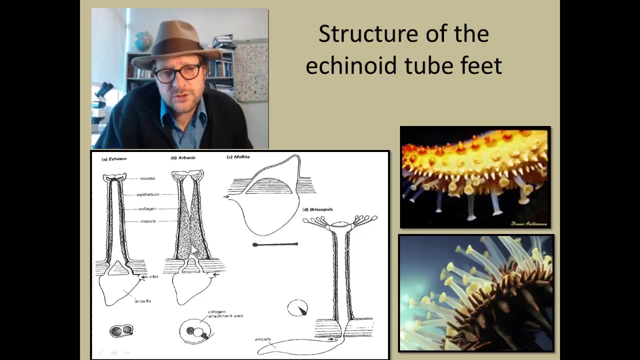 which works as a canal system for the body fluids that pump down into the tube feet. Hence, locomotion is controlled by a vascular system of body fluids that connects with the external ocean water. Each tube feet has an ampulla, a sac, which can be inflated and push water into the tube. 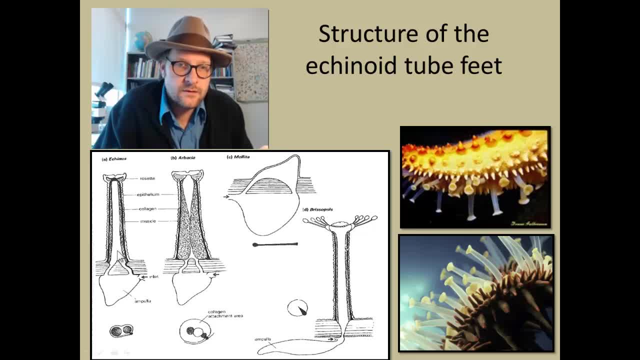 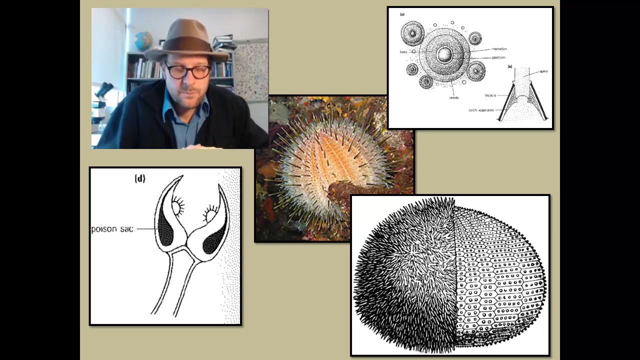 making it more rigid, while at the same time filling the tube with oxygenated water that can aid the muscle tissue on either side of the tube feet. Tube feet also exhibit suction cups, which help the echinoderm to grip surfaces tightly. Icnozoans cover themselves with protective spines to keep predators from taking a bite. 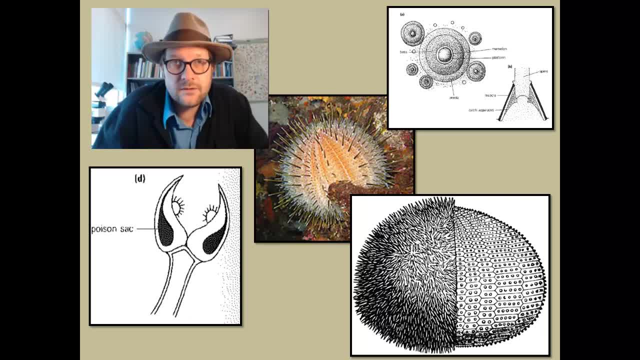 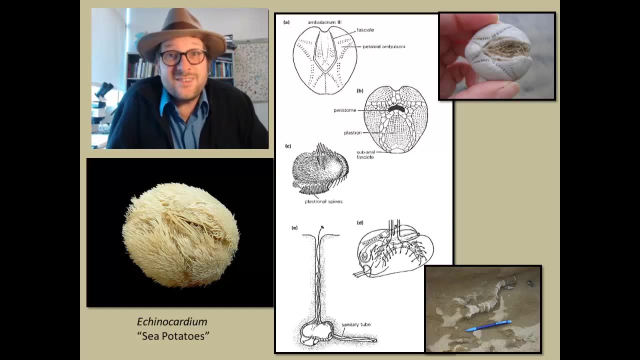 and from other animals from attaching onto their bodies. The spines can be poisonous and can move in response to predators, a bit like porcupine quills that can regrow if lost in defense. One of the most bizarre Icnozoans are the sea potatoes. these are creatures 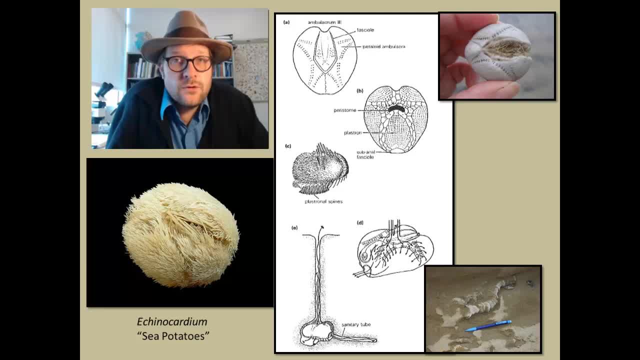 that live in the sea, completely underground, filtering out food using their extended tube feet. They lack lanterns as adults and use their tube feet to acquire food in their burrows. They leave behind complex traces that can be identified in the fossil record, since 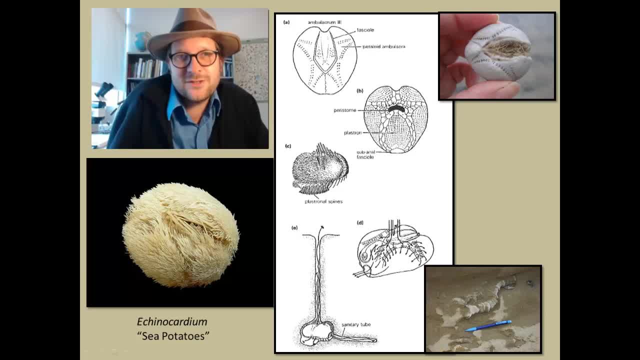 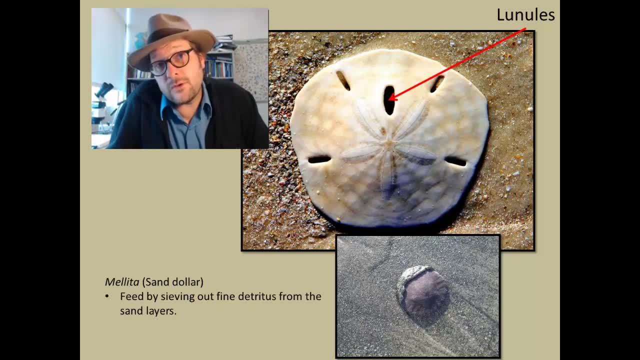 their skeletons are often found within these burrow-like structures. One of the echinazoans that is more familiar to you is the sand dollar, the genus Melalita. These echinazoans crawl through the sediment, filtering out food, and are common in the 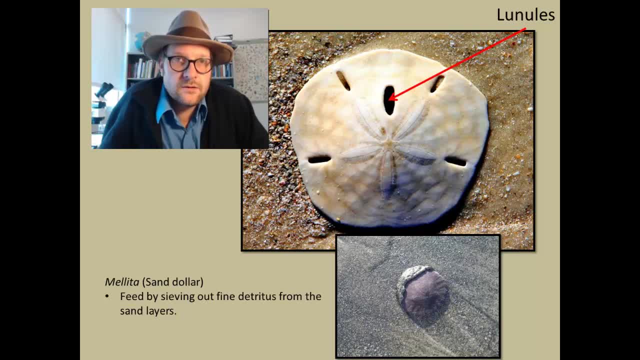 littoral zones along the coastlines. The sand dollars have five perforations called lunals. These lunals help sediment to pass through while food is drawn along the coastline. The echinazoans have long grooves on the bottom of the sand dollar to focus food into. 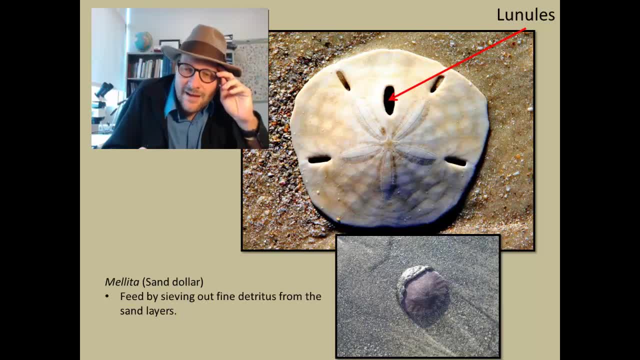 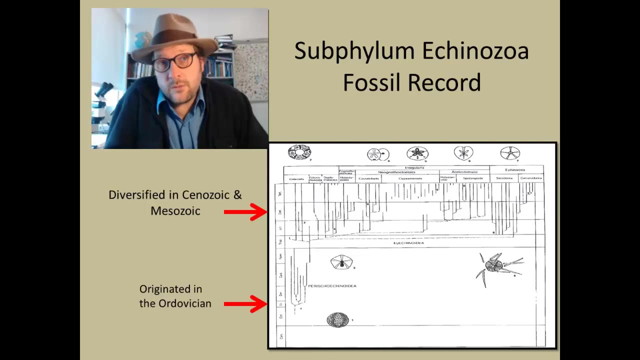 the mouth. Hence sand dollars are adapted to a specialized food-gathering adaptation in sandy sediment. The echinazoans originated during the Ordovician and often are grouped into whether they are irregular, that being, whether they are bilateral or regular, in which they exhibit five-point. 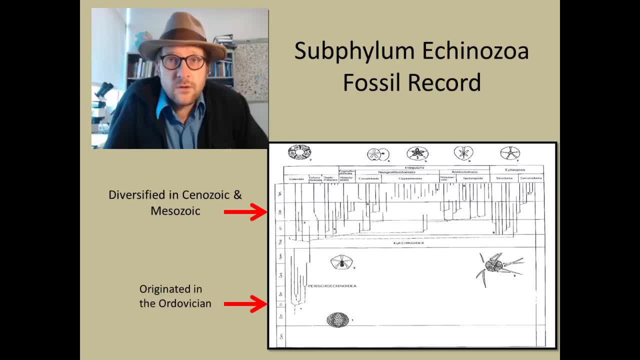 symmetry. One interesting feature of the fossil record is that echinazoans become diverse as you get into the Jurassic and Cretaceous and particularly are diverse in the Cenozoic. In fact, today they are a very diverse group and doing quite well. 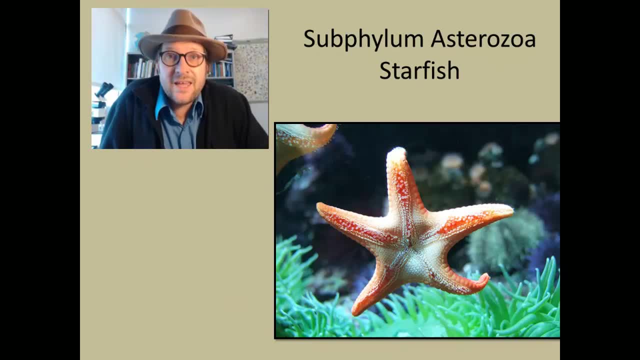 The next subphylum are the astrozoans: the starfish and brittle star. They differ in having five arms, although some can divide these as well to have multiples of five arms. With a very pentagonal body plan, Each arm is flexible and can move around the ocean floor. 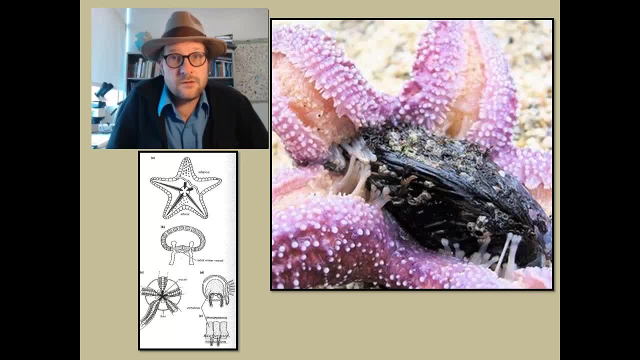 Astrozoans are predators of many shelled organisms that live on the sea floor and they use their podial feet to crack open shelled organisms. These starfish can invert its stomach in the shell and they begin to digest the shelled organism. 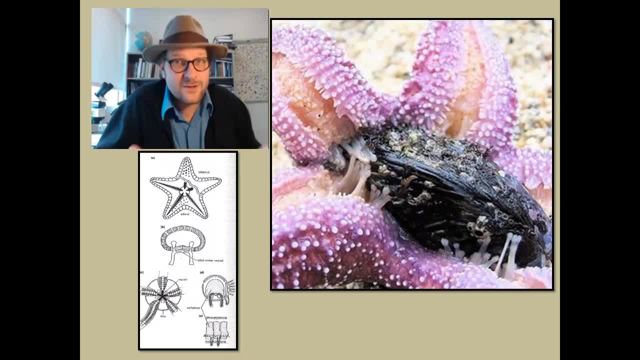 This type of feeding is very successful and astrozoans are numerous in many locations where there are plenty of shelled organisms for food. They don't require large amounts of food and they have a very slow metabolism, allowing them to coexist in many marine ecosystems. 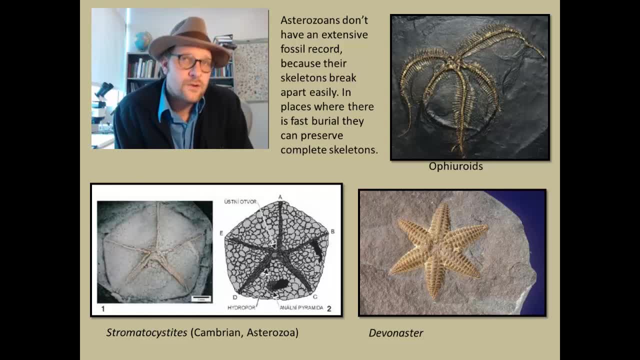 Starfish don't preserve their fossils as often as other invertebrate groups, in part because their arms are rather brittle. They easily break apart. The earliest starfish are found in the Cambrian and they lack the five arms but still retain. 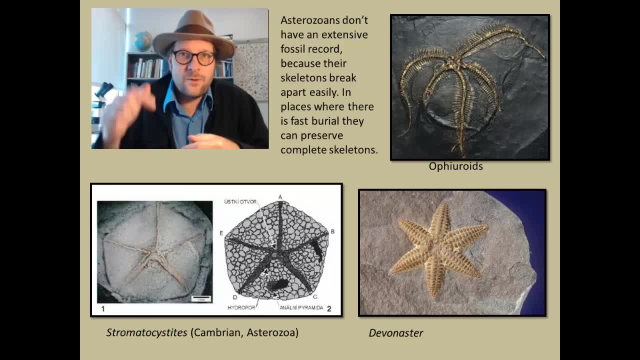 a pentagonal body plan instead. For example, the early genus Stromatocytes lacks the characteristic arms but still retains a five-sided symmetry that characterizes later members of the astrozoa. Some beds have a five-sided symmetry. Some beds have a five-sided symmetry. There are many other species of starfish that have been found that preserve a lot of starfish which have been rapidly buried and several rock layers around the world preserve wonderful starfish in fossil record. One of those that is fairly common is Devonaster from the Devonian Period. 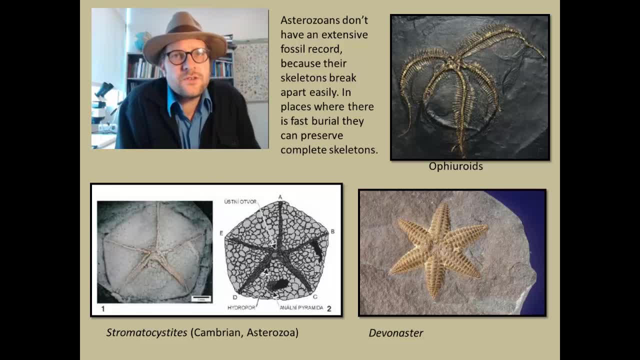 The Ophophores are the brittle stars and they have much more slender, flexible arms. They first appeared in the fossil record during the Ordovician and are still living today. Next we come to the Great Fossilized Group. 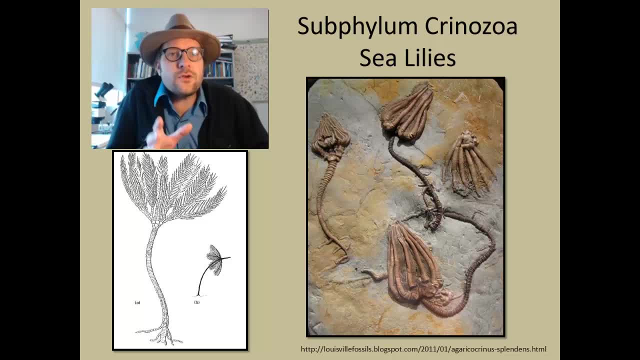 group, the crinozoan or the crinoids. This group was once called the palmatazoans or stocked echinoderms, since, rather than being mobile, they remain sessile on the ocean floor Today. they include the sea lilies found in many marine environments. 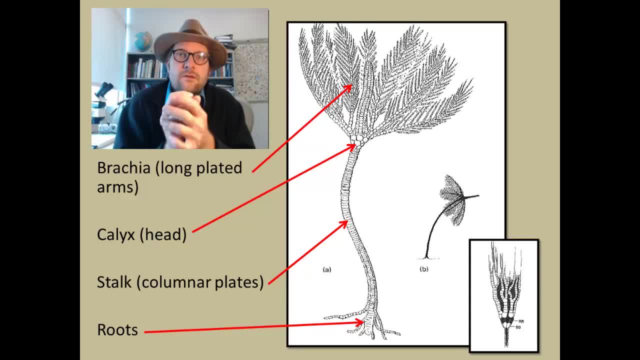 The anatomy of the crinoid body is divided into the brachia. these are the long plated arms that wave around gathering food. the calyx, which is where the mouth and gut are present, and supporting the calyx is a long stalk of columnar plates made out of calcite. 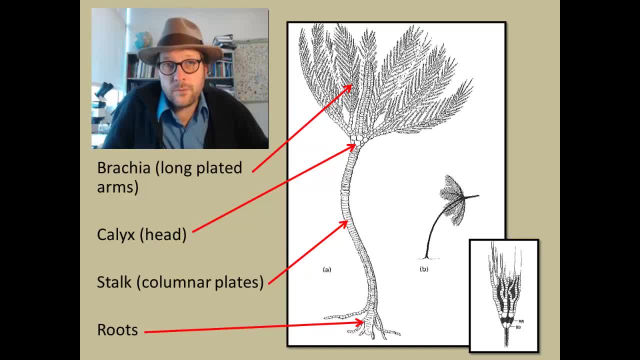 The stalk is akin to stacked coins and does not allow for much movement. At the base of the stalk are the ribs. These ribs hold fast down the crinoid to the sea floor. Crinoids are analogous to a kite tied down by a string on the sea floor and the brachia 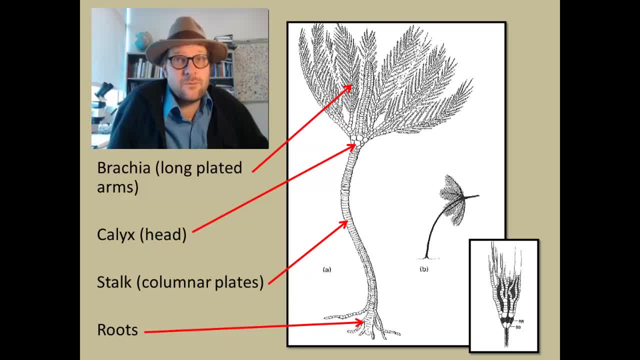 are the mobile parts of the body. Some crinoids may have been more mobile in the past, but were not nearly as mobile as their close relatives, the starfish, sea cucumbers and sand dollars that can move around the ocean floor Despite being sessile. 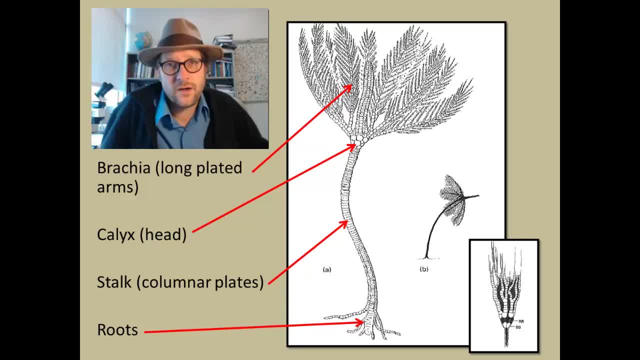 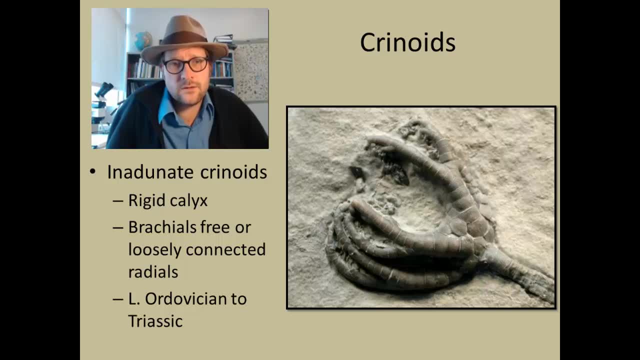 There are four major kinds of crinoids. The first major group is the inordinate crinoids, which have a rigid calyx with brachials that are free or loosely connected to the radial. The inordinate crinoids are known from the late Ordovician to the Triassic. 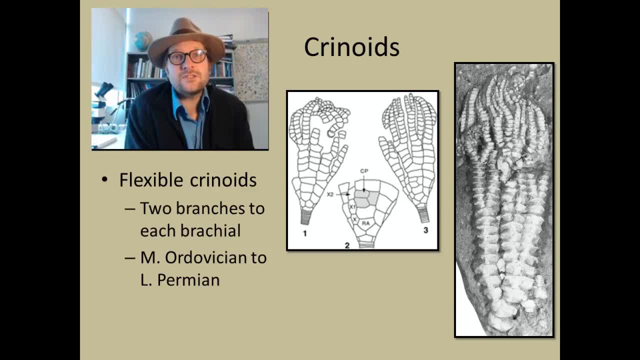 The next group of crinoids are the flexible crinoids. These are the flexible crinoids which have branches off of the brachials, giving them a wider distribution of arms. They are known from the Middle Ordovician to the Late Permian. having fallen victim. 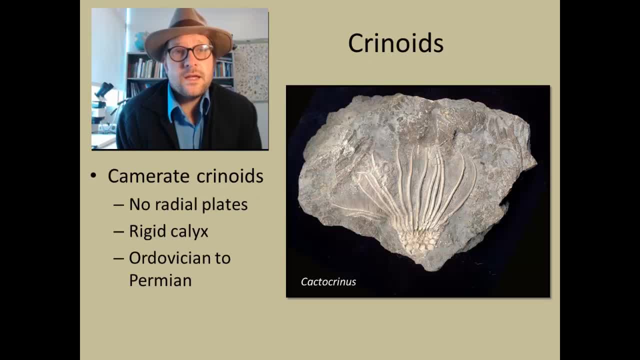 to the Permian-Triassic mass extinction event. The Camarate crinoids are a group which lack the radial plates and have a rigid calyx with many thin brachials. They are the largest group with a fossil record from the Ordovician to the Permian. 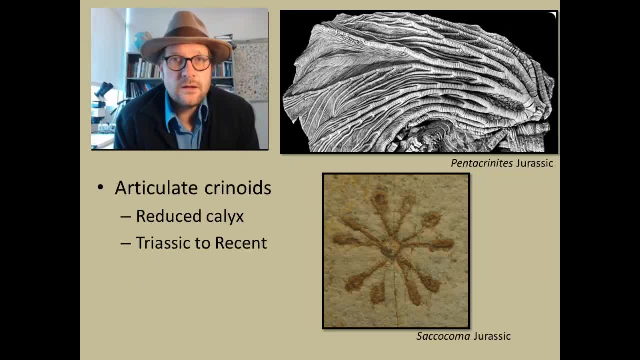 The last group are the articulate crinoids. These lived after the Permian-Triassic extinction and the group that living crinoids belong to. They have a highly reduced calyx with highly flexible arms that can move about freely. There's only about 25 genera today that are stocked, while most living crinoids are unstocked. 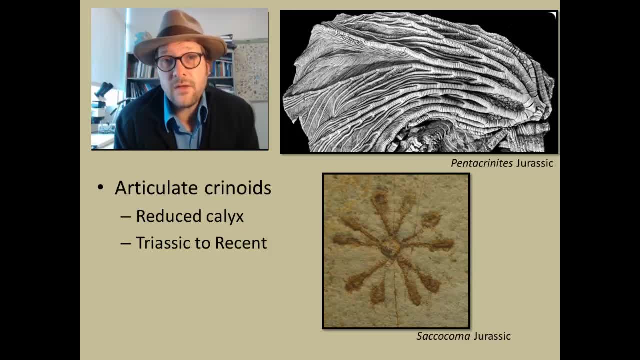 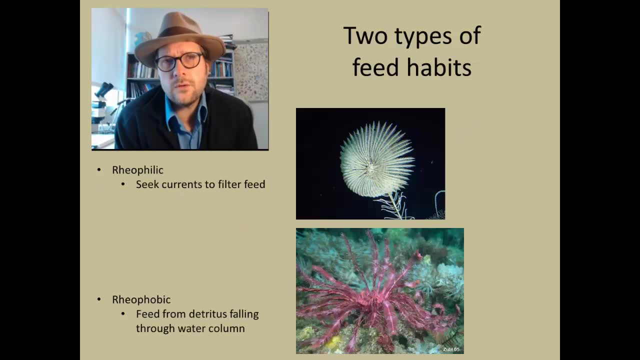 comioloids. These are what is also referred to as the feather stars, and they have roots but lack the columnar stalks. Living stocked crinoids exhibit two different types of feeding, either being renophilic, meaning that they seek out fast currents to filter feed, or renophobic, where they feed. 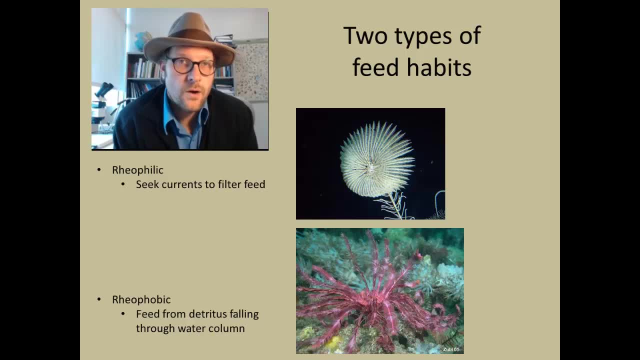 on detritus that is slowly falling through the gentle waters. These two styles of feeding can be good indicators to paleontologists about the flow of ocean currents. Crinoids are really great for reconstructing water flow and currents of the ancient past. 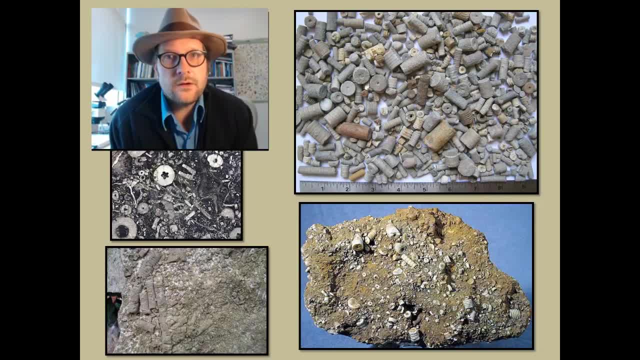 Crinoids are extremely common in the fossil record, but rarely do the calyx or brachyels preserve. Most often is the columnar plates which, when examined along the transactional surface, exhibit a five-pointed star. These fossils also resemble stacked coins and can be found in many fossils. 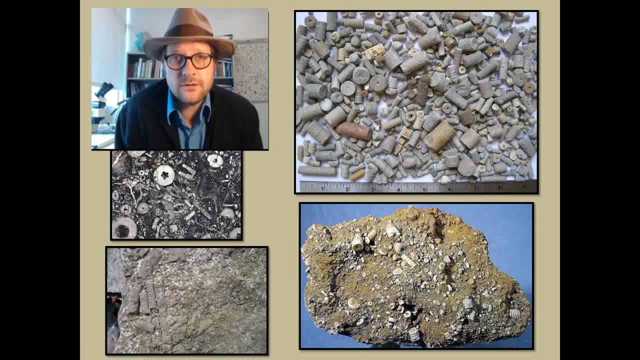 These fossils also resemble stacked coins and can be found in many fossils. Crinoids are extremely common in the fossil record, but rarely do the calyx or brachyels preserve. Crinoids are extremely common in the fossil record, but rarely do the calyx or brachyels. 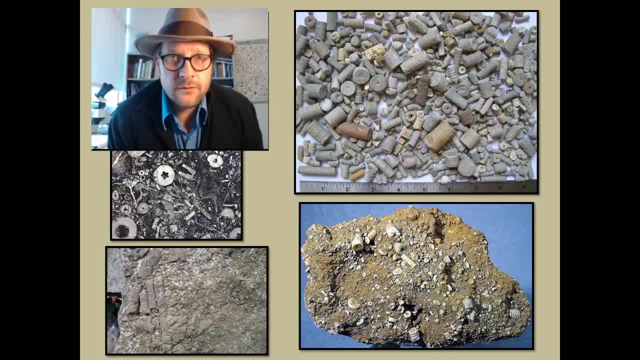 preserve Most often is the columnar plates which, when examined along the transactional surface, exhibit a five-pointed star. These fossils also resemble stacked coins and can be found in many fossil collections, Because it is often the columnar stocks that are preserved. we don't necessarily have 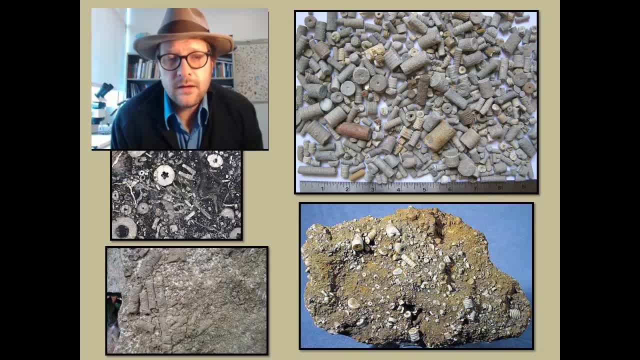 a complete picture of what the living crinoid might have looked like, until we find that calyx or brachyels. However, in many limestones, the crinoid stems make up a majority of the framework of the limestone's calcium carbonate matrix. 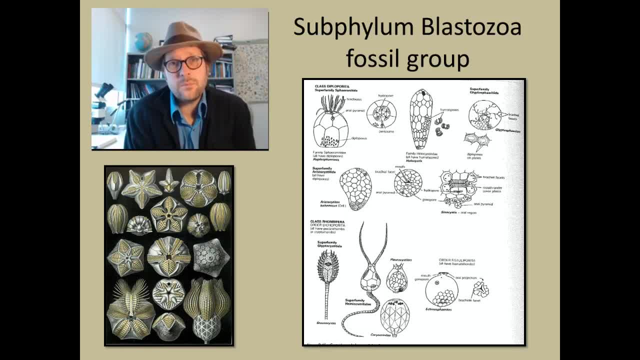 The next group is one of the more bizarre groups of enchinoderms, The blastozoans. These only preserve the calyx portion of the animal, or theca, In life. these creatures had short stalks and tiny brachyels used to filter food much. 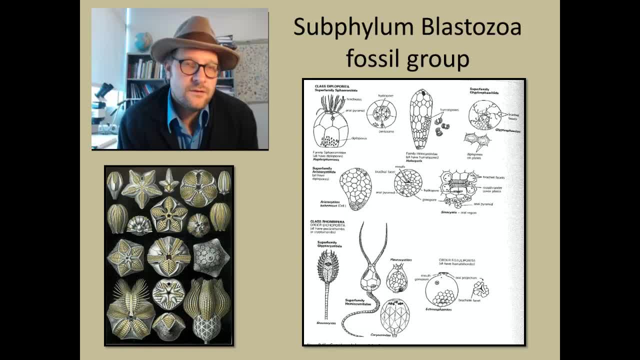 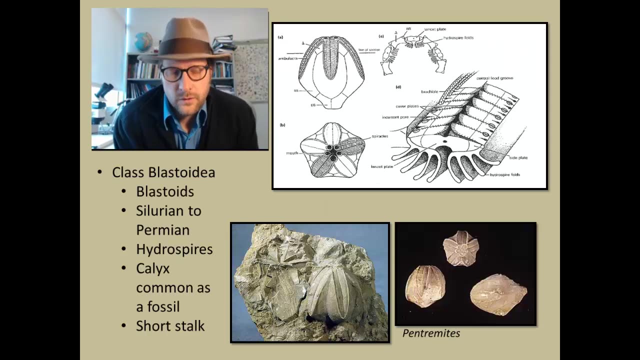 like crinoids, However, these structures lack calcite skeletons and hence are rarely preserved. What is preserved is the bizarrely complex theca which served as the major portion of the body structure of these creatures. The class Blastiodia or blastoids lived from the Silurian to Permian, going extinct. 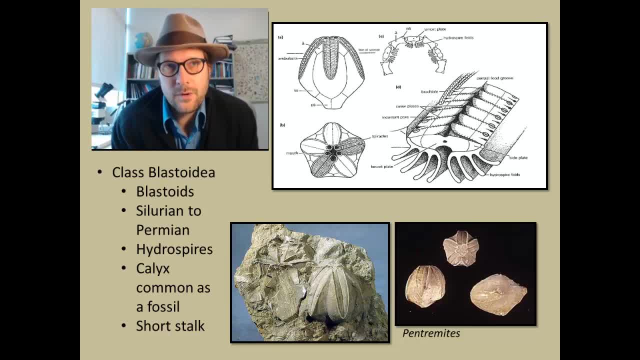 at the end of the Permian-Triassic mass extinction. Their calyx is common as a fossil and exhibit what are referred to as hydrospirals. These spirals, likely, were lined with cilia and beat a current of water to flow past pores. allowing for respiration. 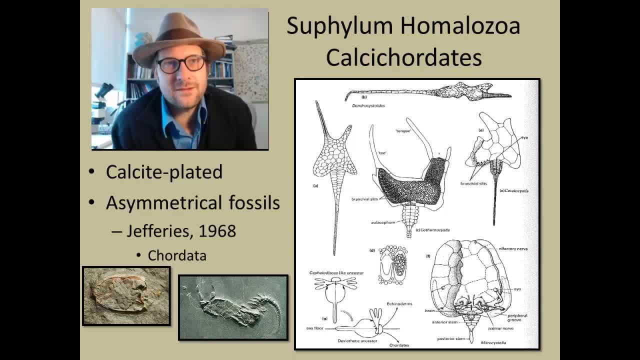 phylum, the homolyozoa or the chalcolchordates. Unlike any other echinoderms, this fossil group, also called the carpoids, are asymmetrical, with a complex skeleton made of calcite. There is some debate of what constitutes the head or tail of these creatures. with some 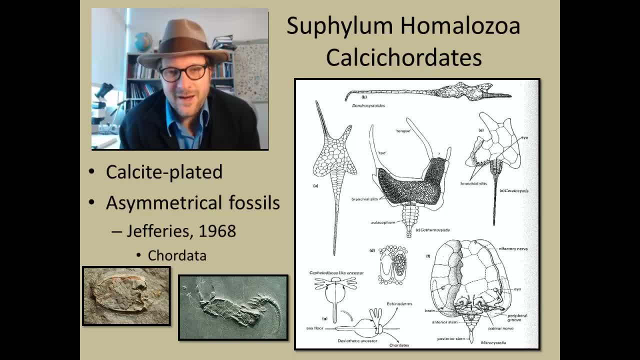 scientists arguing that the head was actually dragged, with the tail being a front leg, or whether they were plunked down and filter-feeding creatures. Some people think that these guys were a bit like a primitive jawless fish and see things that are analogous or synonymous with early chordates, early jawless fish. 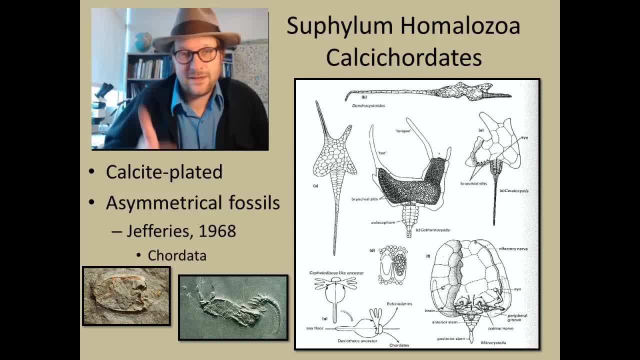 Based on the asymmetrical body plans and the heavy calcite skeletons, these creatures may have had very limited movement and may have acted like the blastoids for filtering food out of the sediment. They are a really peculiar group and are in need of further study to figure out how these 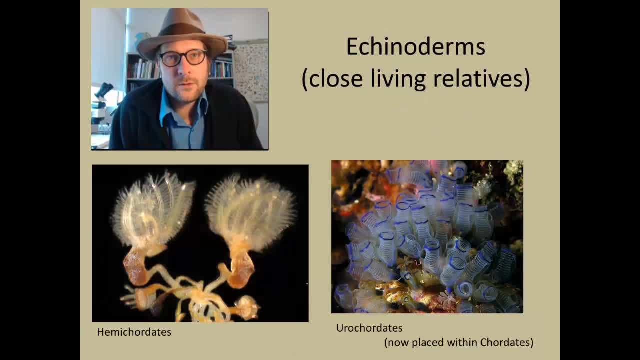 guys were living and behaving. Today we have two additional invertebrate groups that are not well represented in the fossil record. They are sort of inactive. They are in between echinoderms and chordates, the group we belong to. These are the hemichordates and the eucordates, the C-squirts. 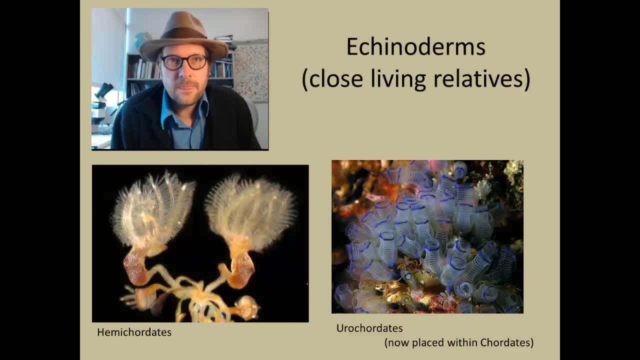 These two groups I discussed in my vertebrate paleontology class, and it may be that these bizarre chalcocordates or hemlyozoas belong to one of these living groups and developed a calcite skeleton secondarily. Now let's quickly go through the fossil record of the various echinoderms again. 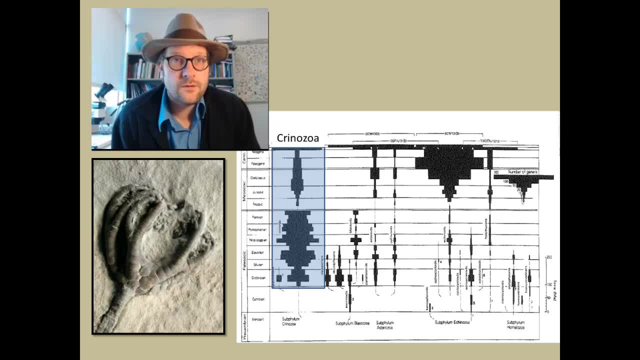 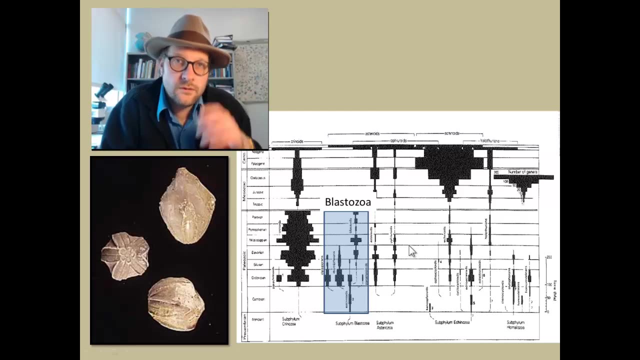 The crinoids originated during the late Cambrian, becoming very diverse throughout the Paleozoic and then undergoing a mass extinction at the end of the Permian Triassic boundary, with a modest recovery since then. The blastozoans originated during the Cambrian, with several groups living during the Early. Paleozoic, with only the blastoids making it to the end of the Permian. they all went extinct at the mass extinction event. The Astrozoans don't have as diverse a fossil record, despite having a fossil record that goes all the way back to the early Ordovician or late Devonian. 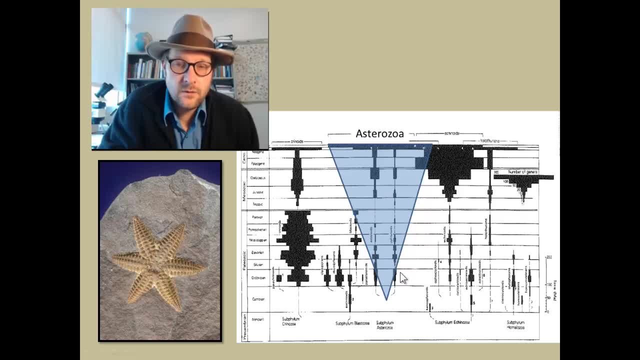 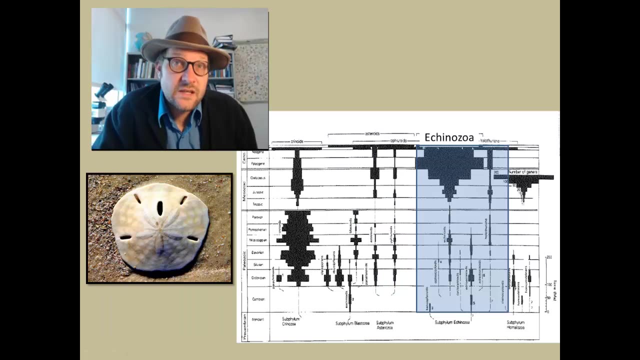 Both the Astrozoids and the Ophians have a fossil record back to this period of time. In all likelihood, these two groups were much more diverse in the fossil record. The Ichnozoans, the sea cucumbers, sand dollars, sea potatoes and sea urchins have a fossil 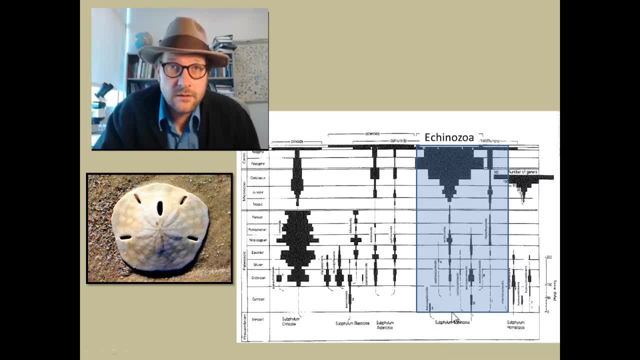 record that extends back to the early Cambrian, but most of the diversity of the group appears in the later part of the Mesozoic, with many of the common forms not appearing until we get to the Cenozoic. The last group is the Homlyozoans, the Chalcocordates. 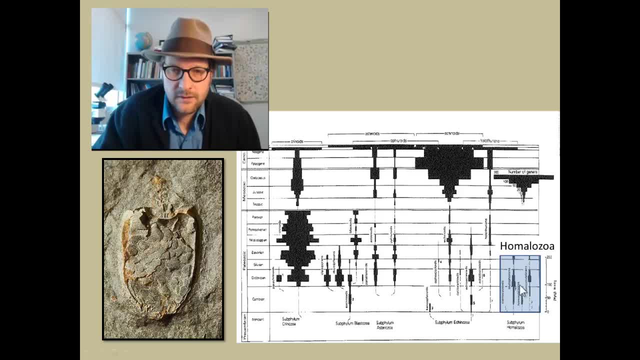 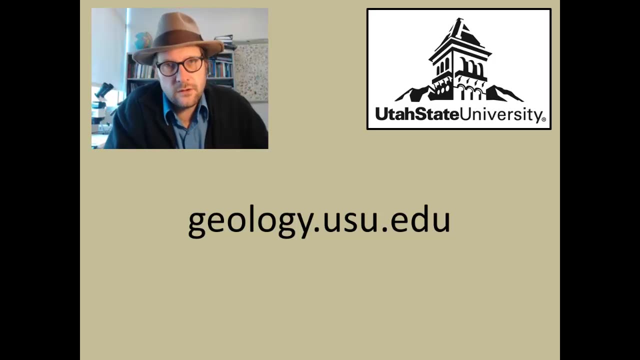 This weird group appears during the Cambrian and extends into the Devonian, and are represented by an unusual primitive stock of echinoderms or related forms. at least Thanks for watching this lecture. If you are interested in taking a geology class at Utah State University, please click. 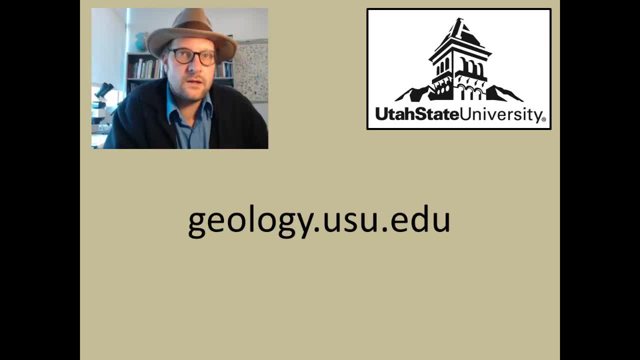 on over to the geology website, geologyedu, And if you are interested in who I am and the research that I do, come stop by my website at benjaminslashbergerorg. Thanks again for watching. 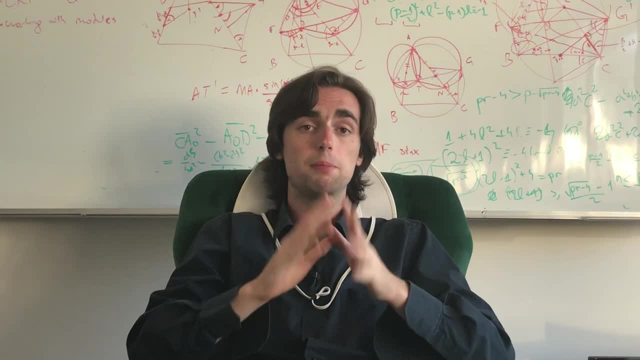 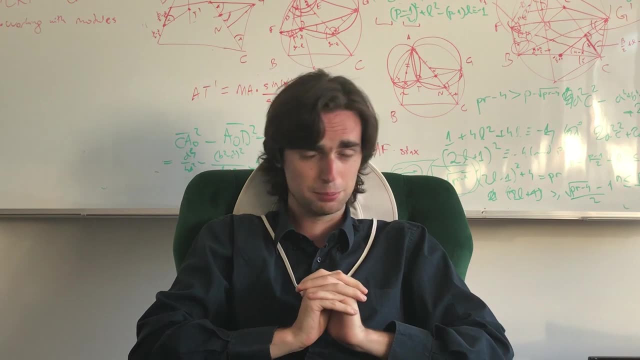 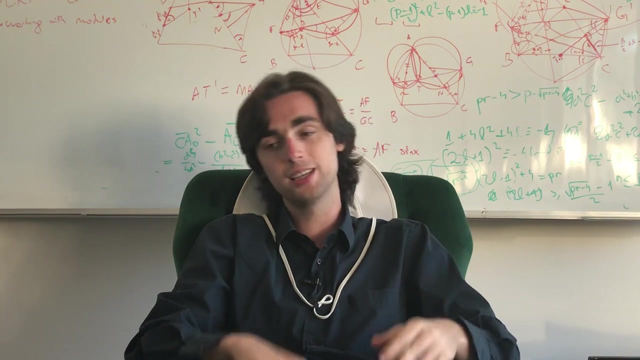 Hello, fellow problem solvers. So today we're going to be talking about what you need to learn- do to learn- number theory for the International Math Olympiad. So without further ado, let's begin. There's really two paths here. One path is the path of solving problems from number theory and the other one is reading different books, textbooks, handouts and the like. 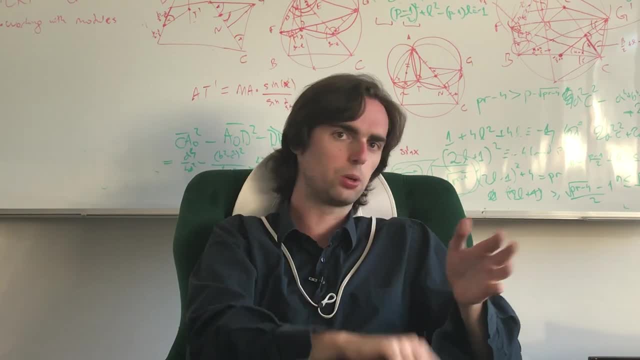 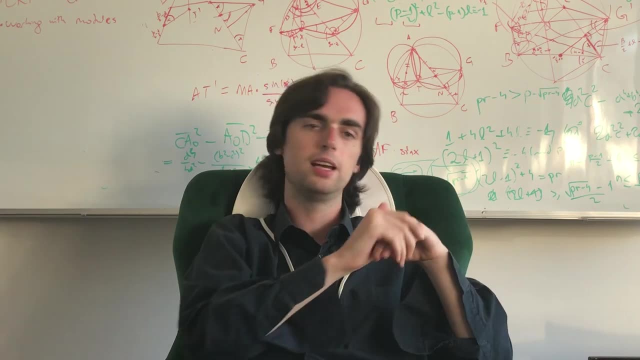 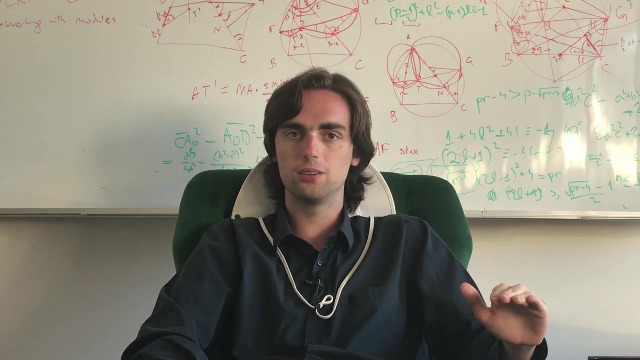 So solving different problems, it's always the same story. Start looking at problems at a level of a competition that you're comfortable with and move up. If you pick a competition that's too hard, try to, you know, take it a level down a notch, take another level down. 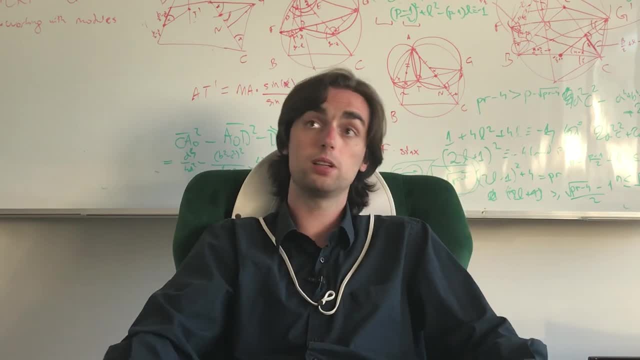 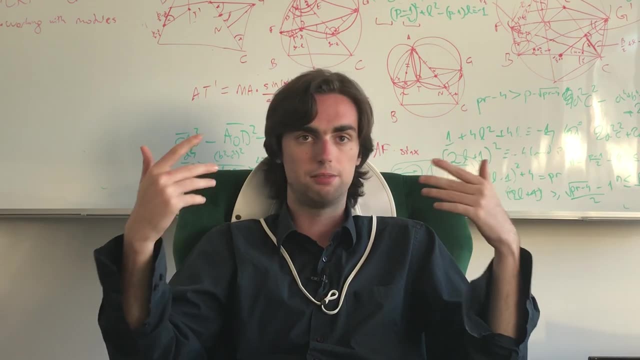 So if you're trying to solve a problem from the IMO, you can't solve it. well then, try to solve a problem from Romania team selection test. If that's too hard, try to solve it from the IMO. Try to solve the Romania's junior Balkan Math Olympiad team selection test. 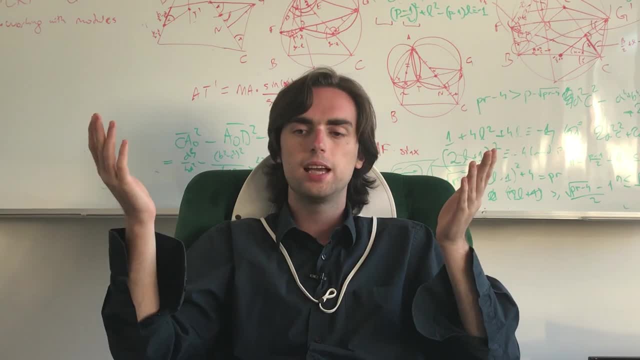 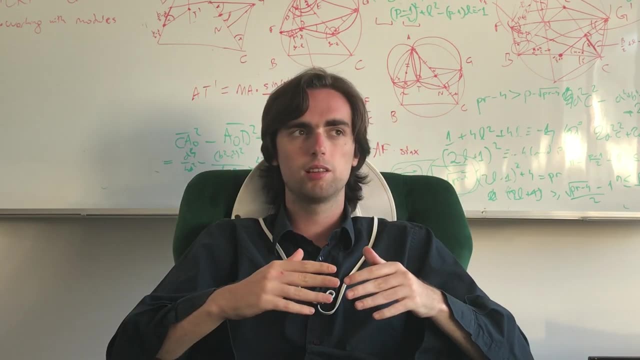 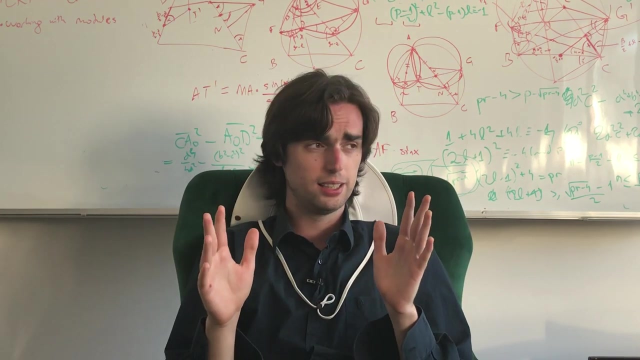 If that's too hard, try to solve an 8th grade problem from Romania, Like, try always to go down and down and down until you're comfortable solving your problems. So that's one. But with textbooks, really, the only thing you need is there are many different textbooks available and I can't really recommend any single one.